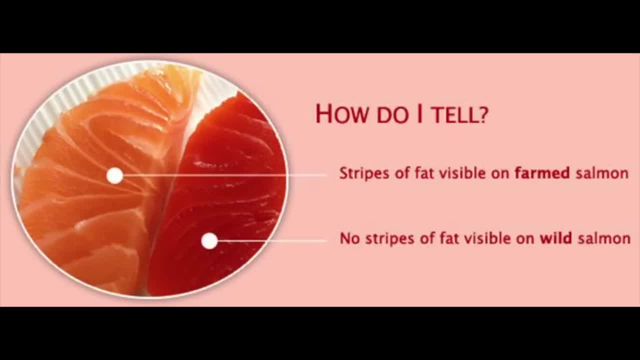 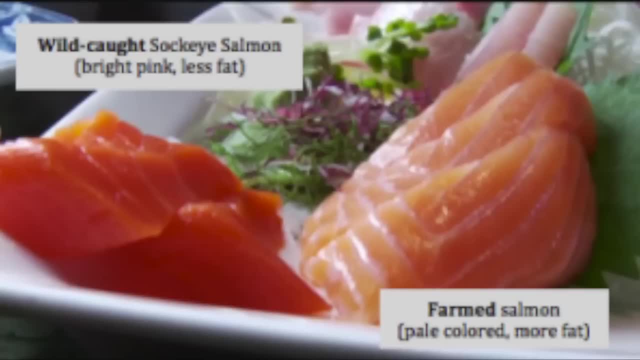 Farmed salmon is on a very, very controlled diet. They can manipulate the color. they can tune in and dial in with the salmon feed. okay, with those pellets, The salmon food is tuned in and dialed in and has dyes in it. 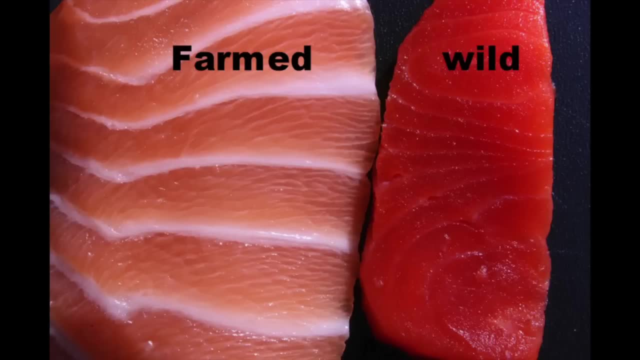 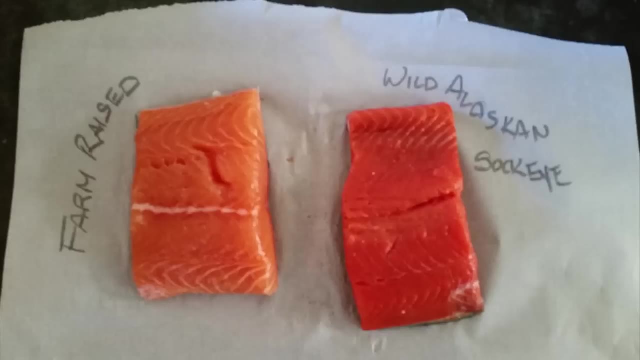 And if they didn't dye, the put dyes in the food, The salmon would not be pink or orange like it is. it would be a very grayish color. Certain fish, and especially salmon and trout as well, take on the color of the pigments. in their diet. When I was in Colorado, when I had a restaurant in Colorado, we used to buy trout- farm-raised trout- from a local farm- very, very small, only had three or four ponds they were raising in super awesome operation. 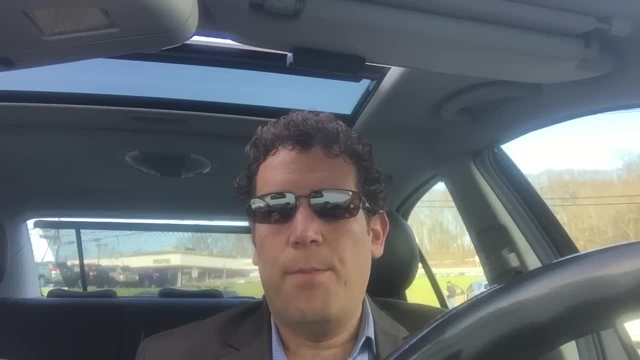 And every now and then trout would come in pink. We'd get pink Pink trout. So this was way back in my culinary career and I said to the lady. I said I know it's in their diet, but can you explain this to me a little further? 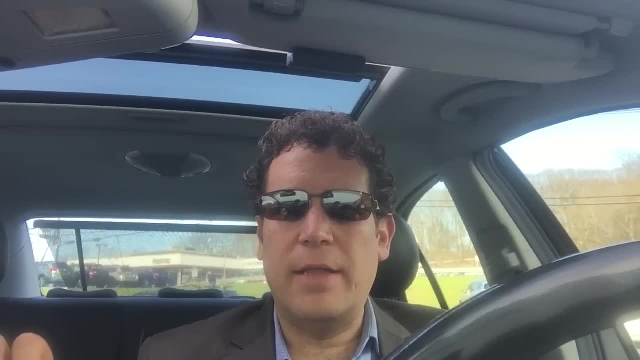 And she goes. sure, Marcus, She goes. the one pond that we have has this freshwater crustacean. a freshwater shrimp is in this pond. The fish eat that, and thus it turns the pigment of their skin. They're eating this pigment, it turns their skin, and so when you get fish that have this, 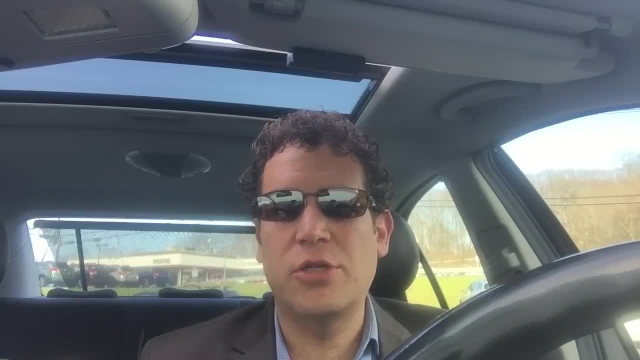 this pinkish, orangish tinge on the flesh. she goes those come from a specific pond in the farm that only has this, only has this type of shrimp, only has shrimp, wild freshwater shrimp. And I said, oh, very cool. 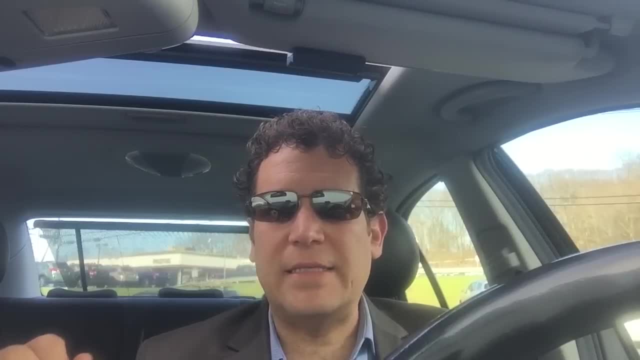 That's what I had figured. So salmon gets its wild. salmon gets its color from the things it eats, like krill, okay. And krill eat a ton of chlorella and chlorella has anisacin, which is a carotenoid. it's. 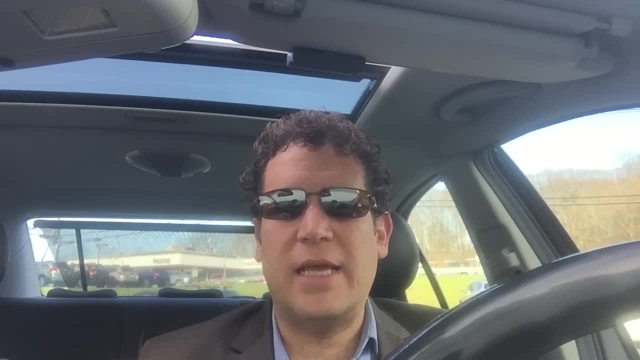 an antioxidant slash, carotenoid, That then translates down the food chain and turns the flesh of the salmon orange. Now I know some of you might say: well, certain salmon isn't orange, it's white. And those are in very, very rare cases where you get king salmon, wild king salmon from. the Pacific Northwest. they call them albinos or ivories, and those fish are indeed white or ivory-fleshed salmon. A lot of people think that's a delicacy. they love it. It sells for much of a higher price. I would suggest, if you ever see it out there, try it. If you're a salmon eater, totally try it. It's an interesting product. Some chefs will get that in. But other than that, all wild salmon, besides that small, small amount of albino salmon. all the salmons are going to come out, not the same pinkish, orangish, reddish color. They're going to vary based upon species, based upon time of the year, their diet and just you know. those are the factors. And that's the reality of it. So, sockeye versus coho, two totally different colors, versus king versus chum. There's about five or six species of wild salmon on the West Coast, and all these different species are different sizes and different, slightly different colors. So if you're buying king, wild king salmon and all of a sudden you switch to a chum salmon, to a Kida salmon- they're going to be different colors- And all of a sudden you get a sockeye and it's bright, bright, bright. that's just a. 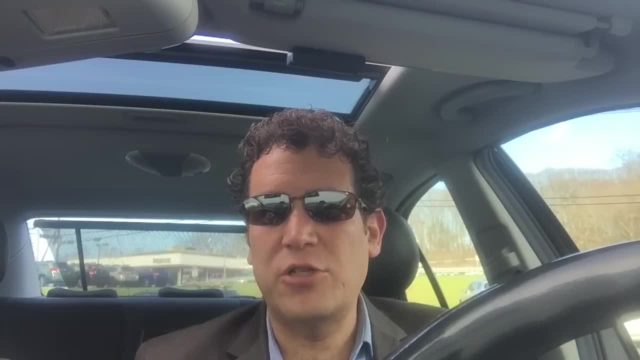 variety of species differentials. okay, So just because the wild salmon is not the same as a farm salmon. see, this person's worldview was different. This person only knew that, hey, I've been eating farmed Atlantic salmon, farmed salmon. 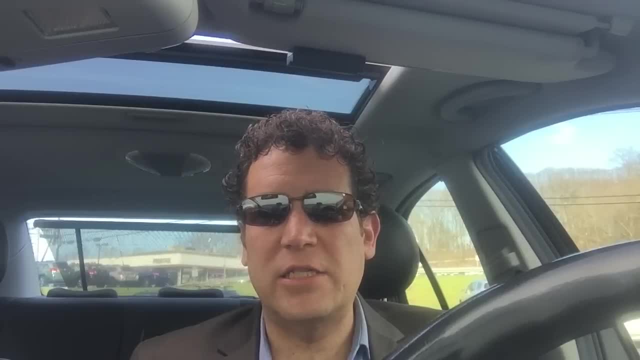 for all my life, and this is what it should look like, this is what I'm used to, this is my worldview of it, so anything else must not be right. In actuality, it's the opposite. The farm salmon is the one that has the chemicals, the dyes, the fake carotenoids, or they add. 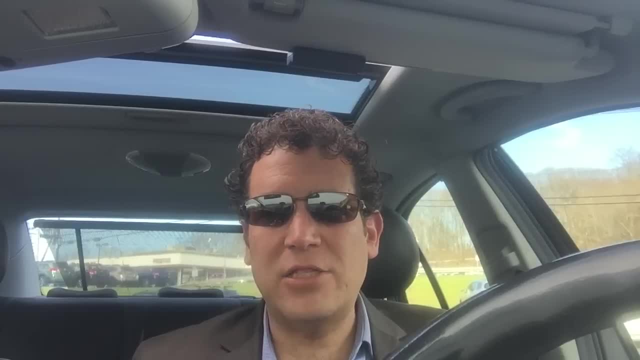 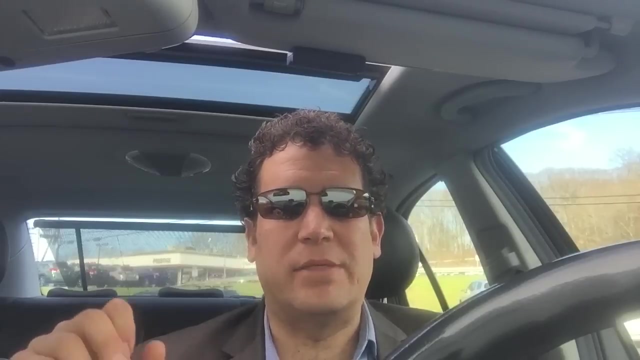 carotenoids to the diet, the pigments, the colorings. that's the one where they've actually manipulated and controlled to a certain extent, where they get it to be the same every time. So it's a consistent, exact, precise colored product and it's the same size fish. they can tune into when it's harvested and, of course, what they're selling to the grocery store, to the restaurant, is: This is a 9 to 12 pound fish. this is a 12 to 15 pound fish. this is a 15 to 18 pound. 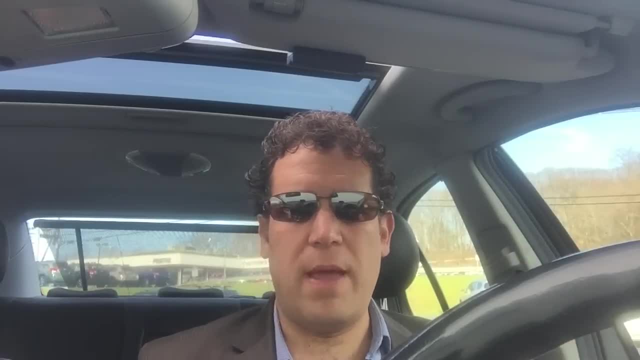 fish. they can dial those in and just say this is it. and here you go, bam bam, bam, bam. same color across the board. So the consumer who's been consuming this is now confused when they switch to a wild. salmon that's eaten, a natural diet that has tons more nutrients, much more omegas- I shouldn't say much more omegas- because they've again tuned or dialed in the feed of the salmon, where they boost the omegas up, but they've also boosted the fat. 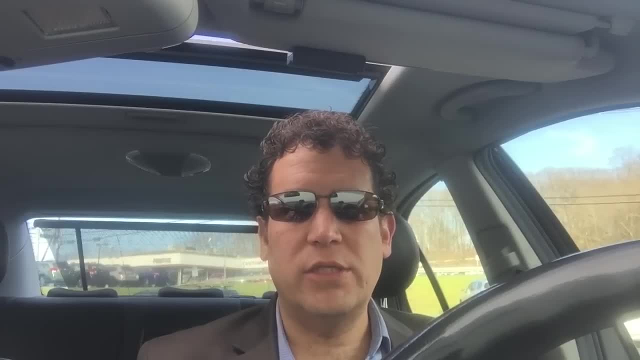 Fat content way, way up. and they've also boosted the PCBs, the dioxins, all that, that, the contaminants way, way up in this fish, because all those contaminants are typically fat soluble, so they stick in with the fat of the fish and the more the fish is fatter. 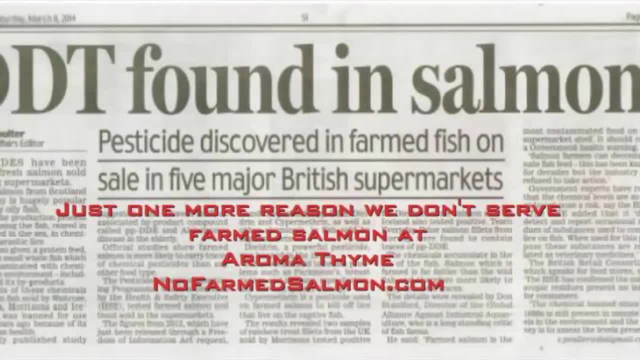 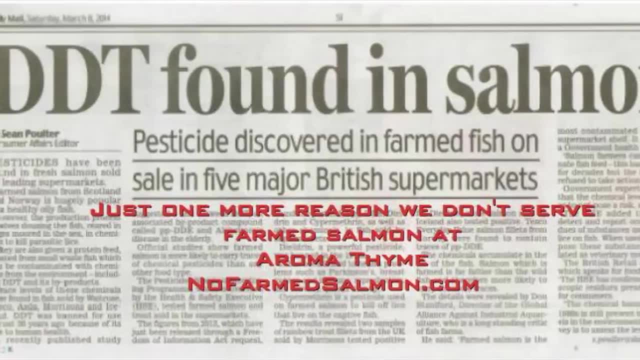 these farm fish, the more contaminants it has. This has been proven over and over and over again. in fact, there's certain countries in Norway and stuff. they've put out notices, doctors have put out notices, organizations have put out notices and say, hey, 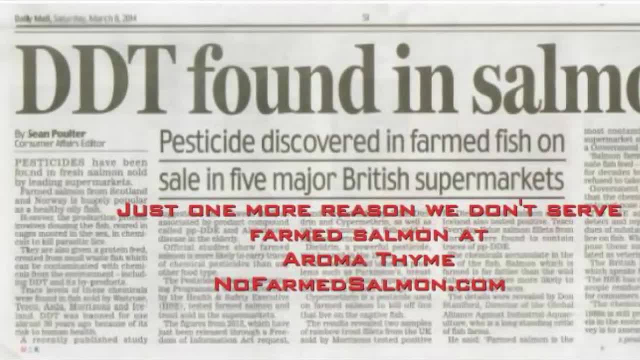 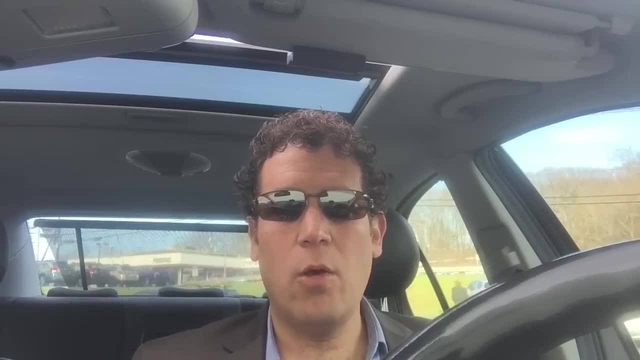 No more than one piece of farmed salmon per month, because the stuff is loaded with contaminants. If you are going to eat salmon, wild salmon is totally the way to go. Go to a health food store. I always tell people: go to a health food store, buy it frozen. Don't go to a fish market unless it's super fresh in season. Your best bet is: go to a health food store. buy the stuff that's wild. go to Whole Foods. go to any other independent, mentally owned health food store that has a great freezer. section and buy frozen salmon. it's super fresh because what happens is they freeze the fish once they catch it. so they catch it on the dock on the boat and it's frozen right away. it's packaged, it has no time to start the aging process because it's frozen. right away and those are super, super fresh. fresher than fresh. don't be nervous that it's frozen. you want to think that it's fresh. there's zero microbes in it. when you defrost it, there are very low microbes.